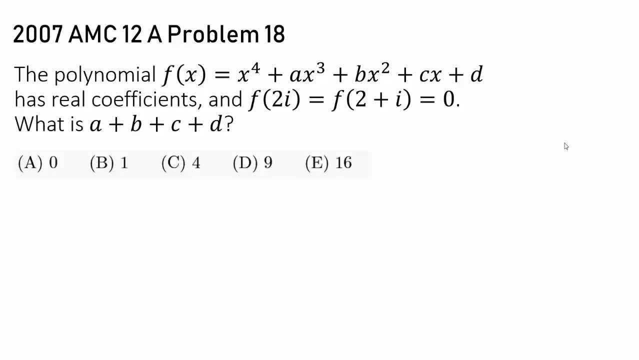 The polynomial f of x is x to the fourth, plus ax cubed, plus bx squared, plus cx plus d has real coefficients And we know f of 2i is equal to f of 2 plus i is zero. So we know 2i. 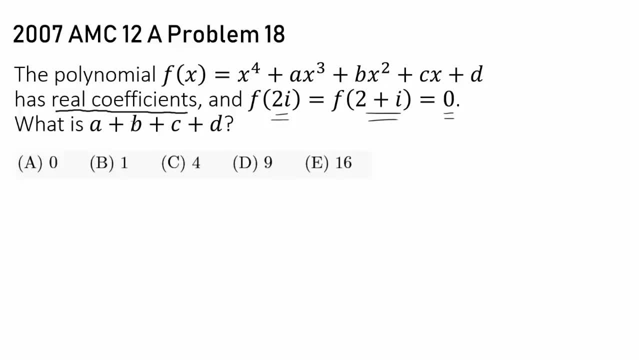 and 2 plus i are the root of this polynomial, And since the polynomial has real coefficients, that's telling us that negative 2i and 2 minus i are zeros as well. So that's what we're starting out with, And we wish to find a plus b plus c plus d. Now, since we know all four of the 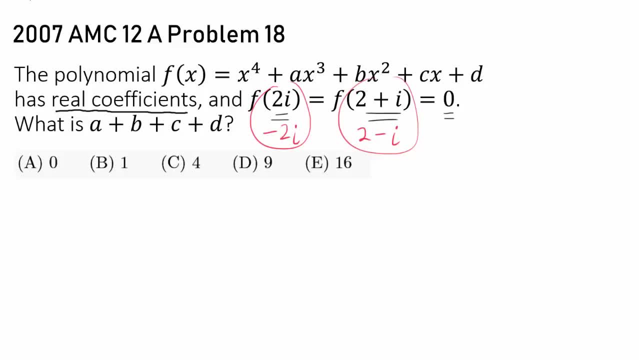 roots: 2i minus, 2i, 2 plus i, 2 minus i. you may say. you may say: if you're adventurous, you can use a Viettas formula. We can use a Viettas formula to separately find a, b, c and d. 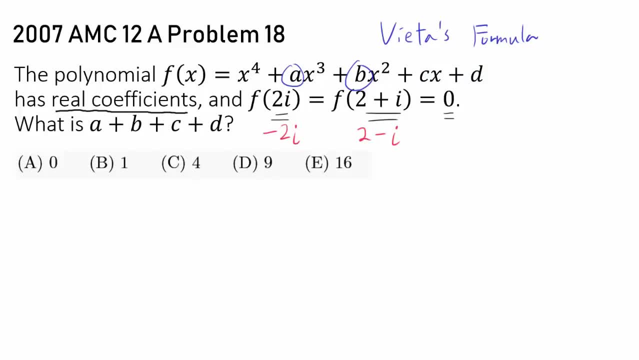 and just add them up, But obviously that's going to take a long time and no one has time for that, So that's not how we're going to approach it. Now, one thing we're going to do is we're going to use a Viettas formula to find a, b, c and d. 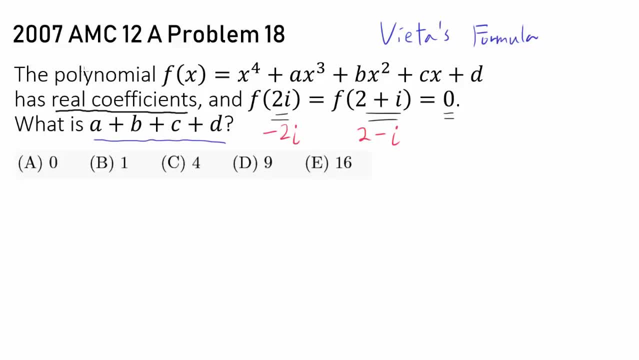 Now one thing I realized when I see this question is that a plus b plus c plus d is very close to the value of f at 1.. Because what is f of 1?? That's 1 plus when x is 1, a plus b plus c plus d. 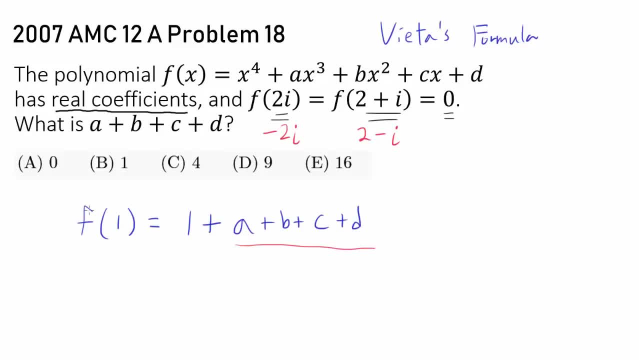 And we want to find a plus b plus c plus d. So once we know value of f of 1, we should be done. But how do you find f of 1?? Well, we know all of these zeros, So we know one way that f of x can be. 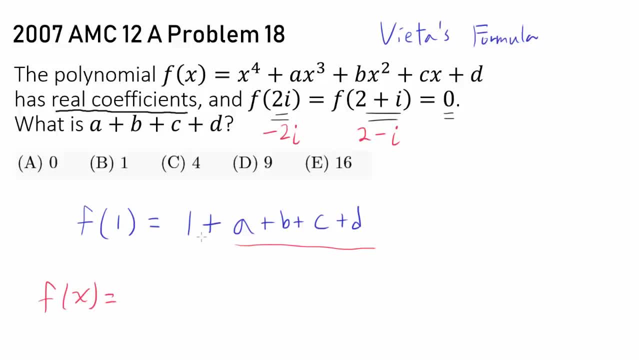 written. We know f of x can be written as x minus 2i, x plus 2i, x minus 2 plus i times x minus 2 minus i, Because you know 2i minus 2i, 2 plus i and 2 minus i are zeros. So you know f can be factored in this form. 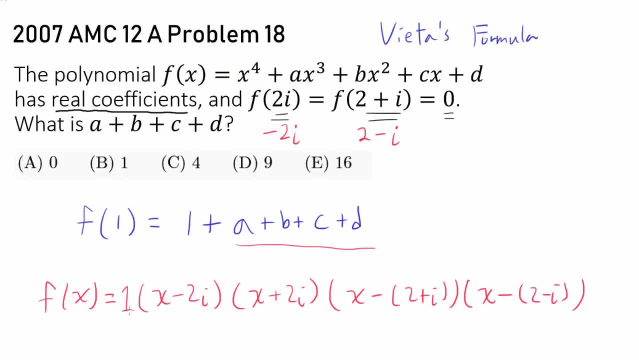 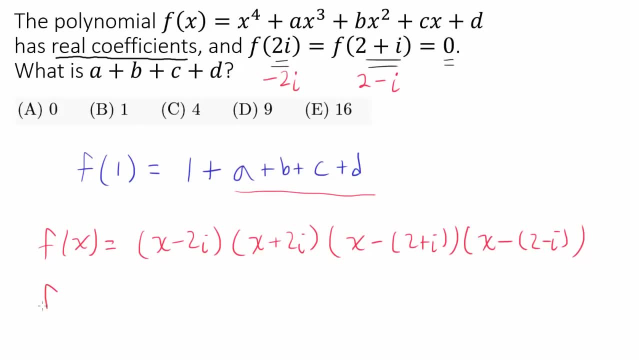 And since leading coefficient is 1, we don't need to put anything except 1 at the front. And now finding f of 1 is very easy, Because f of 1 is going to be 1 minus 2i times 1 plus 2i times. when x is 1, we have 1 minus 2 minus i, which is negative 1 minus i. 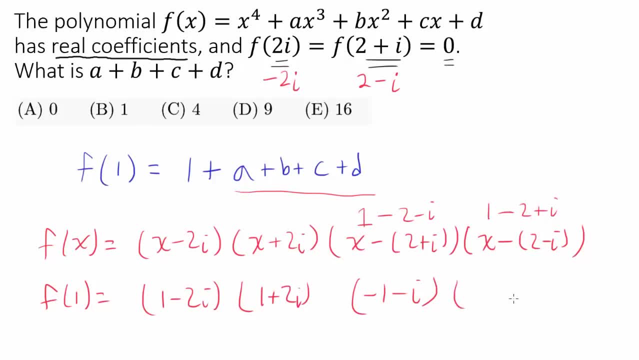 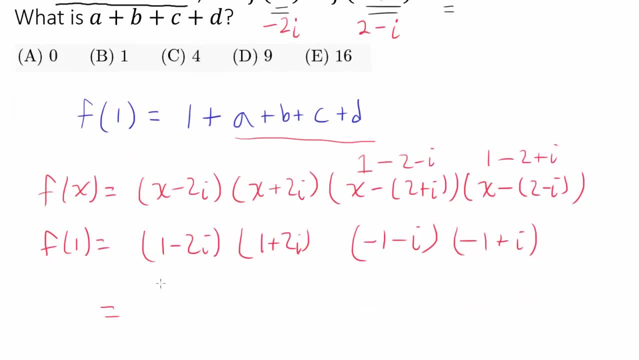 When x is 1, we have 1 minus 2 plus i or negative 1 plus i. And evaluating this is very easy to do: Multiplying these two, we get 1 times 1.. It's difference of squares, So 1 squared minus. 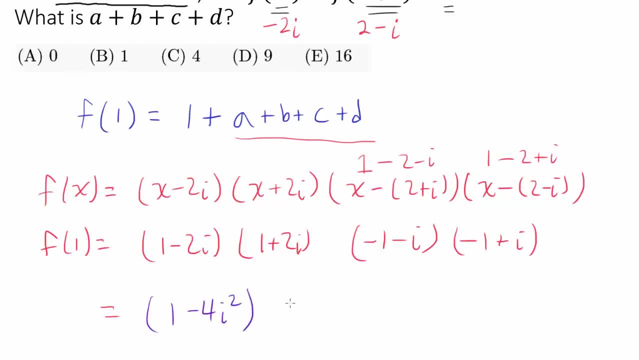 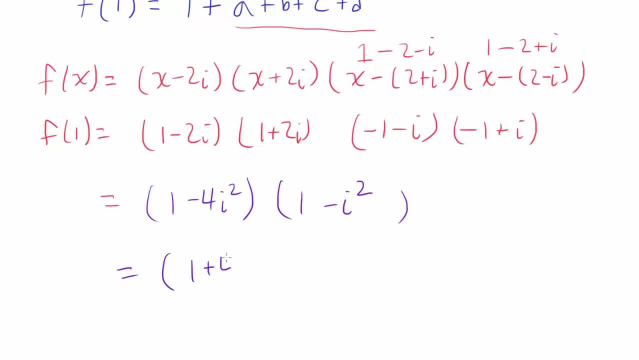 4 times i squared. And of course i squared is negative 1.. And multiplying these two, we get negative 1 squared, which is 1.. And we have a minus i squared, which is, of course, going to be plus 1.. And we see that this thing is 1 plus 4 times 1 plus 1,. 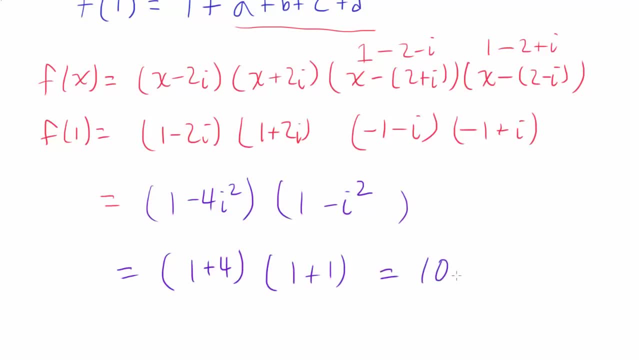 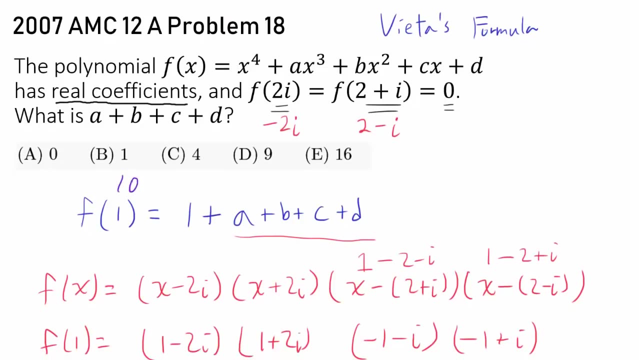 because i squared is negative 1. And that's 5 times 2 or 10.. So we know f of 1 is 10.. So we know 10 is equal to 1 plus a plus b, plus c plus d, And immediately that's telling us that a plus b plus c plus d is 9, or our answer is d. 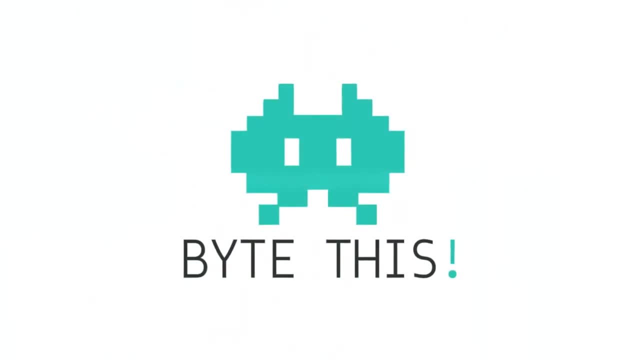 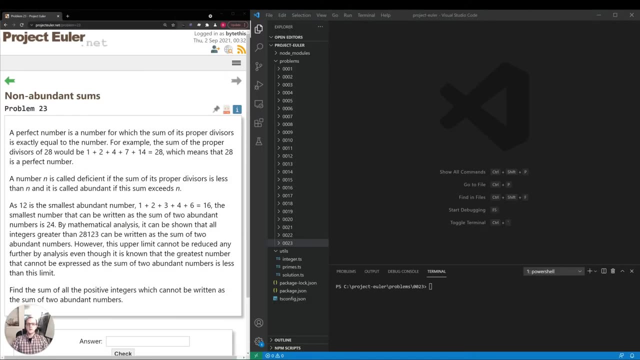 Hey everyone, thanks for joining and welcome to our 23rd video on projectoilernet. Today we're going to be taking a look at problem number 23, non-abundant sums. So the problem reads: a perfect number is a number for which the sum of its proper divisors is exactly equal to the 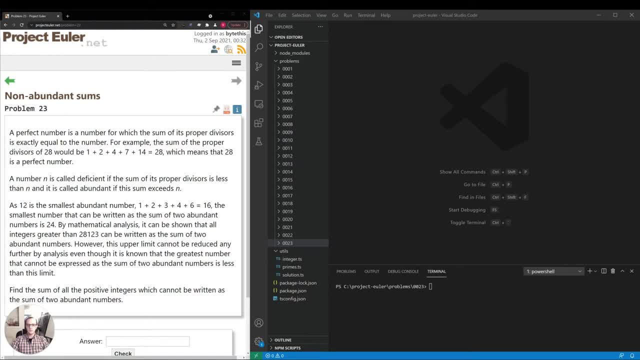 number. For example, the sum of the proper divisors of 28 would be: 1 plus 2 plus 4 plus 7 plus 14 equals 28,, which means that 28 itself is a perfect number. The number n is called deficient if the 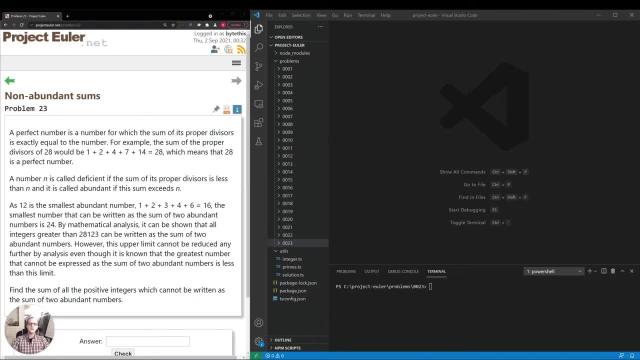 sum of its proper divisors is less than n, and it is called abundant if the sum exceeds n, As 12 is the smallest abundant number. 1 plus 2 plus 3 plus 4 plus 6 equals 16, the smallest number that can.